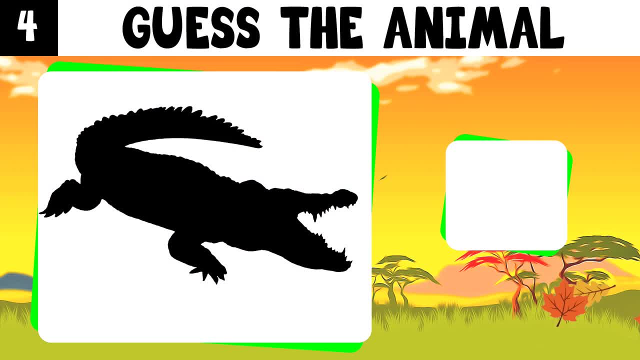 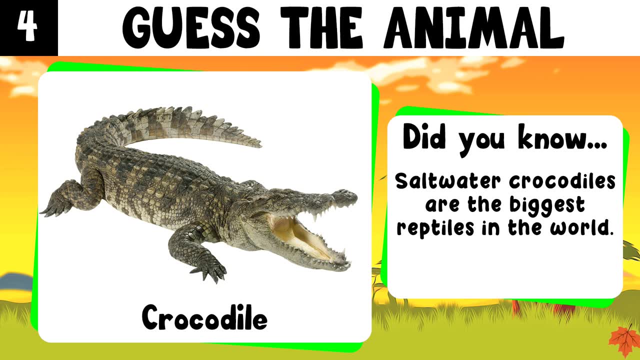 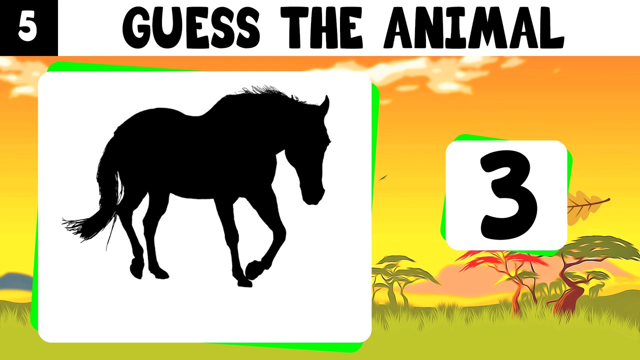 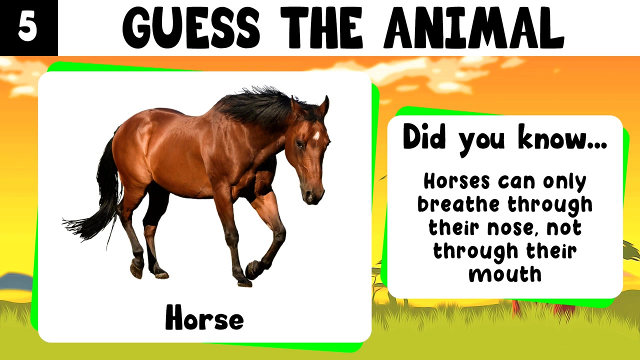 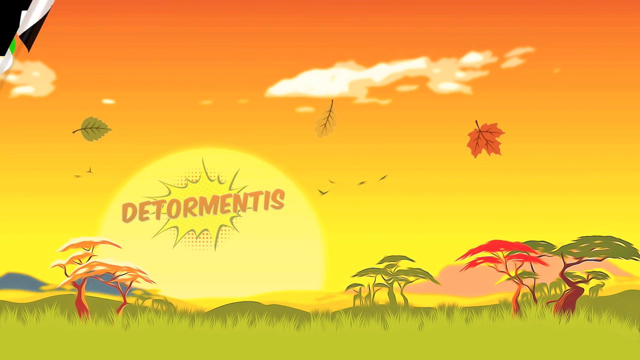 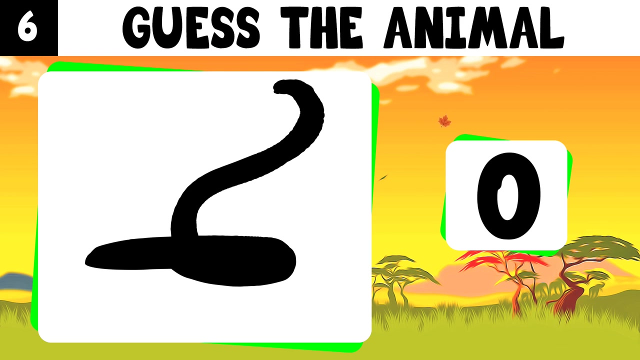 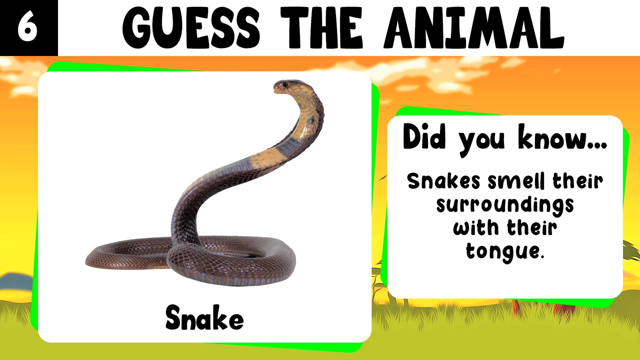 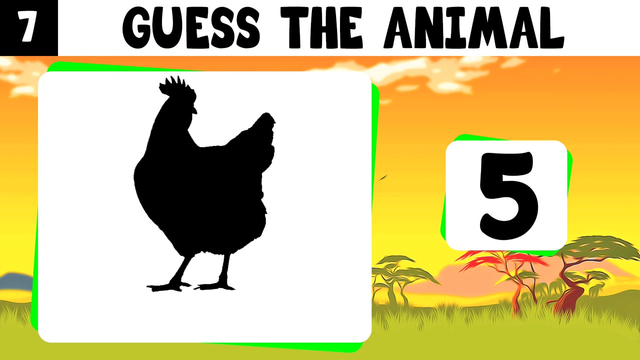 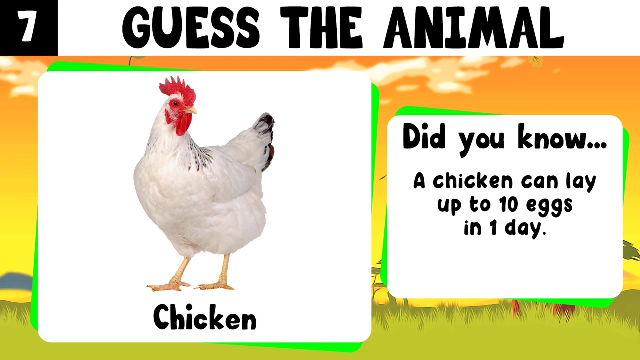 Crocodile. Saltwater crocodiles are the biggest reptiles in the world. Horse Horses can only eat meat. They breathe through their nose, not through their mouth. Snake Snakes smell their surroundings with their tongue. Chicken: Did you know? a chicken can lay up to 10 eggs in a single day. 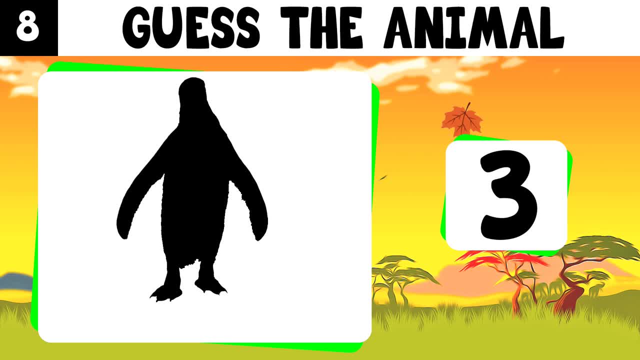 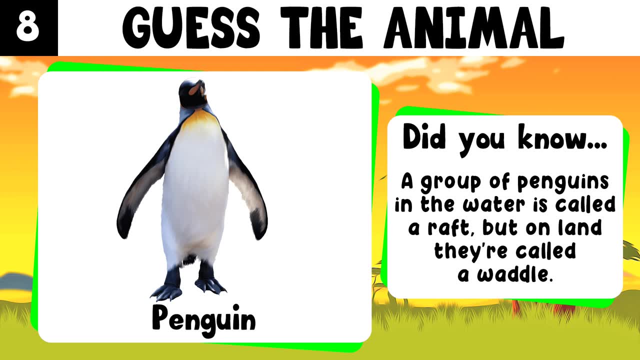 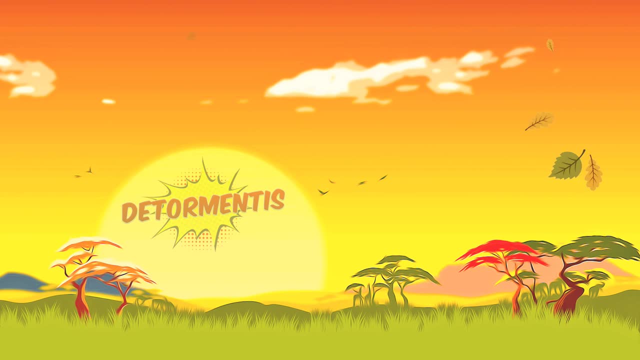 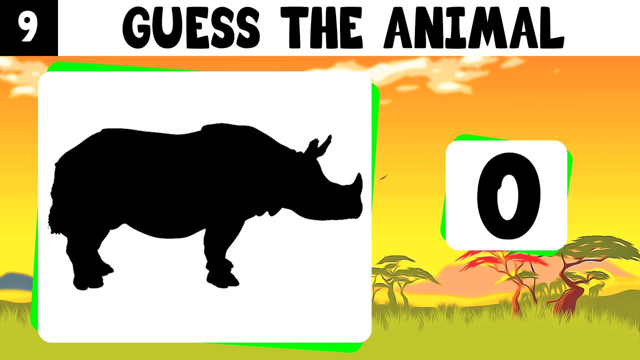 Penguin: A group of penguins in the water is called a raft, but on land they are called a waddle. The only animal that can live in a raft is a leopard. The word is a little difficult to understand. Rhinoceros: A rhino's horn is made from the same stuff as your fingernails. 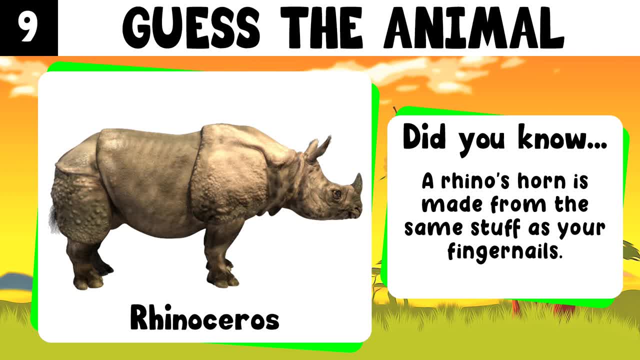 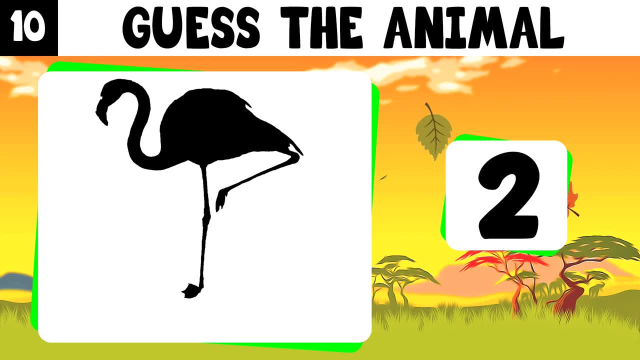 Flamingo. A rhino's horn is made from the same stuff as your fingernails. A rhino's horn is made from the same stuff as your fingernails. Flamingo- Flamingos are filter feeders and turn their 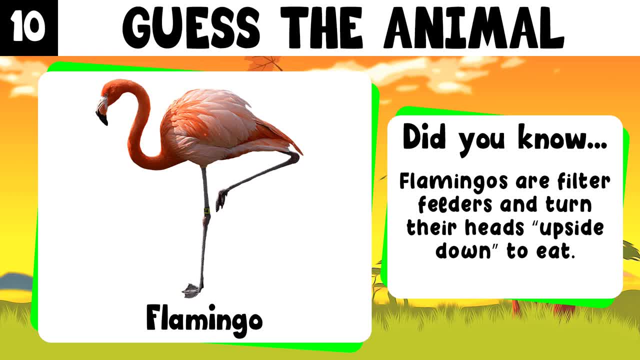 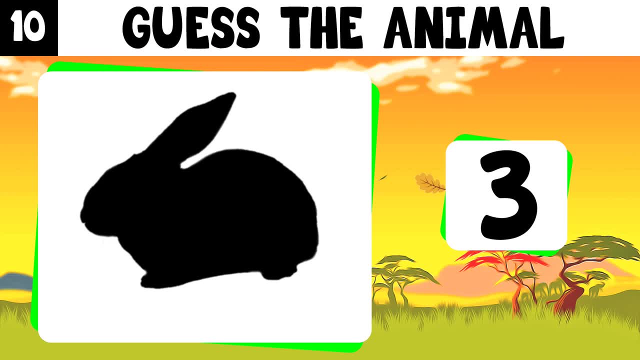 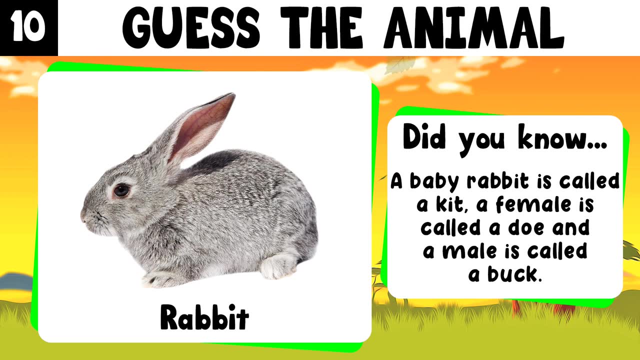 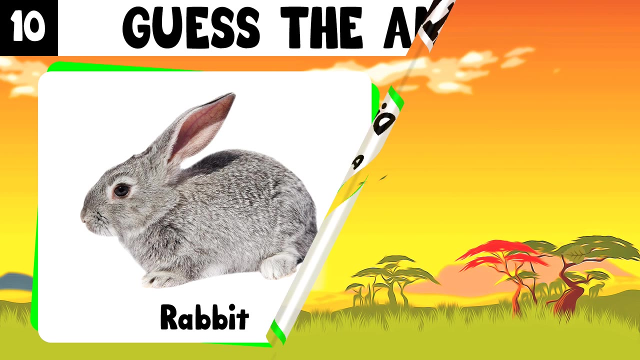 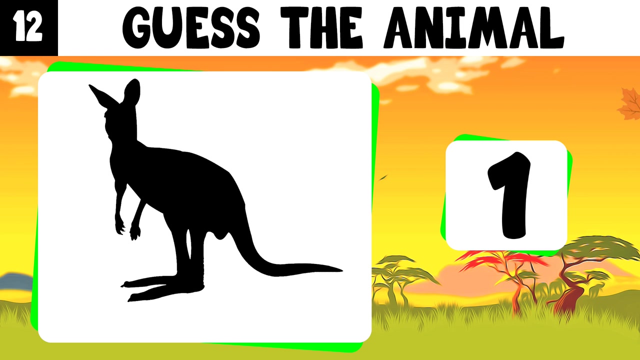 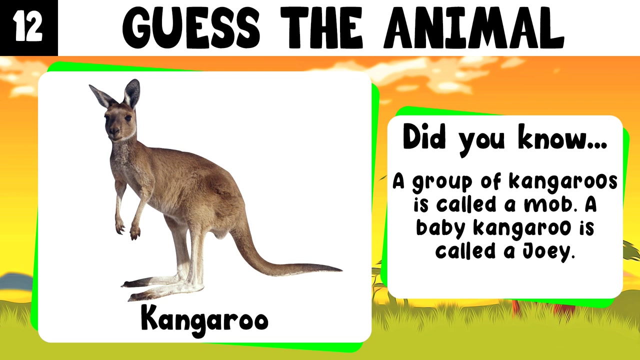 heads upside down to eat Rabbit. A baby rabbit is called a kit, a female is called a doe and a male is called a buck Kangaroo. A group of kangaroos is called a mob and a baby kangaroo is called a joey. 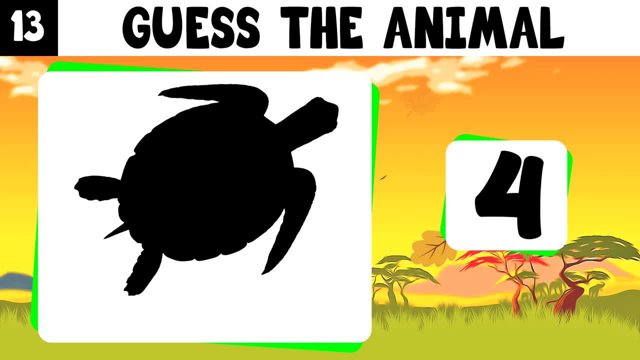 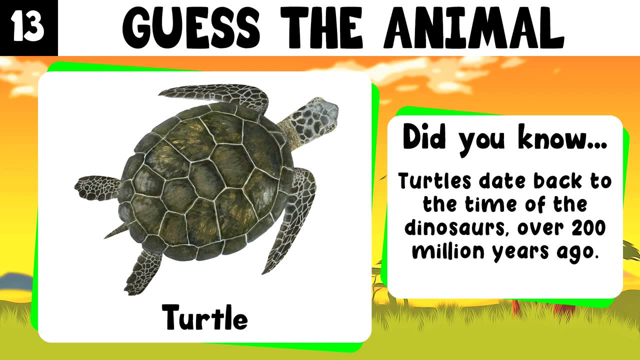 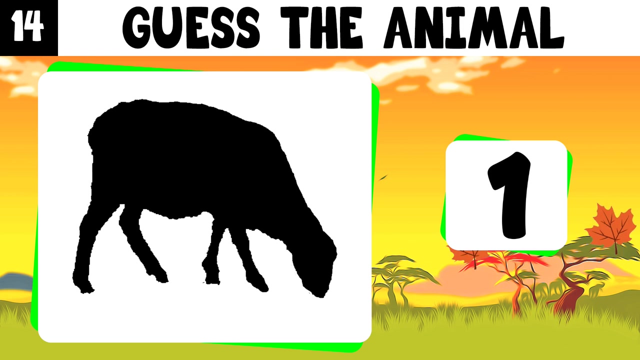 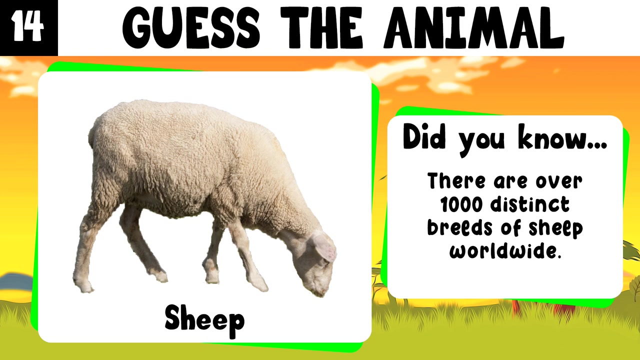 Coyote Turtle. Turtles date back to the time of the dinosaurs, over 200 million years ago. Sheep: There are over 1,000 distinct breeds of sheep worldwide: A female, A female is a male and a male is a female. A male is a female. 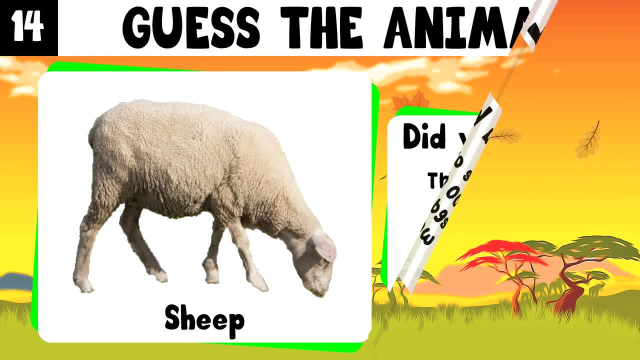 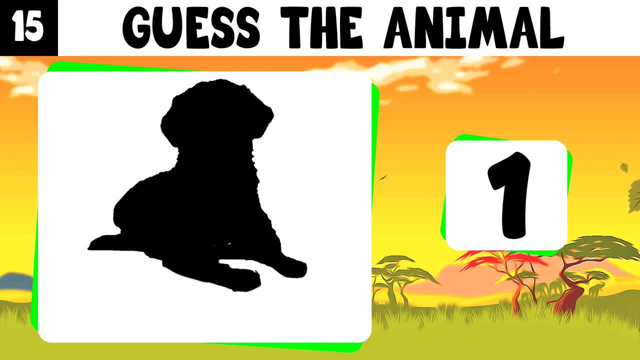 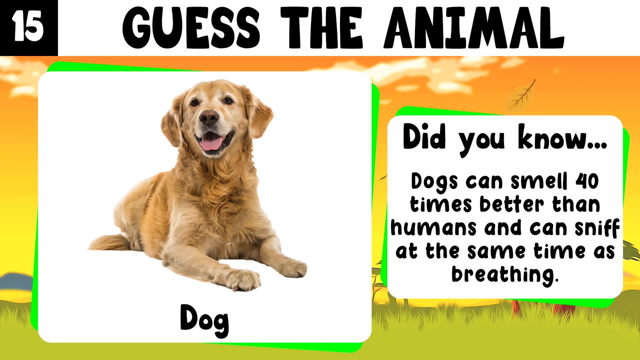 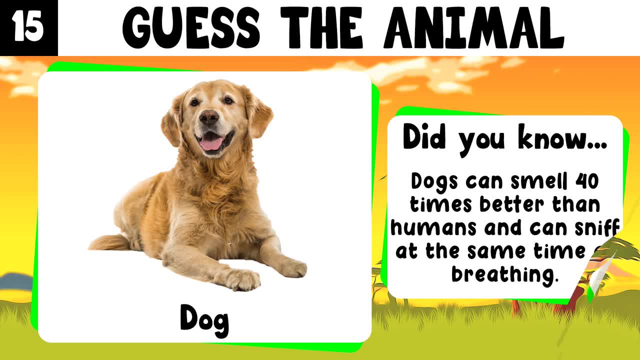 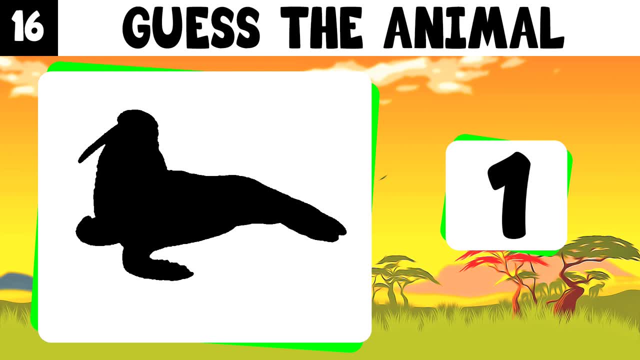 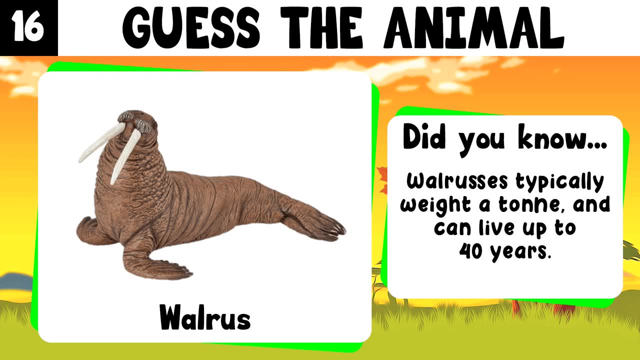 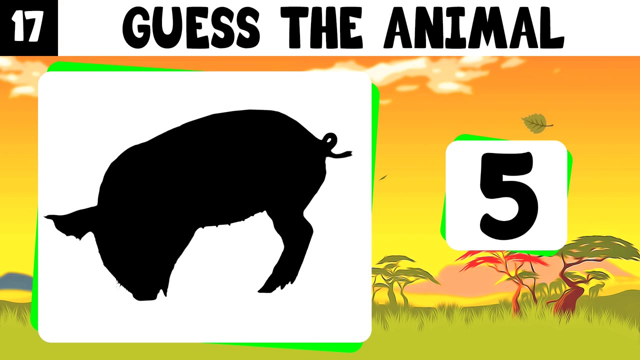 A law is gum. A law is a law is a law. A law is a law is a law. Dog- You can say fresh and natural A". I think dog is a dog, Equally weigh a tonne and can live up to 40 years. 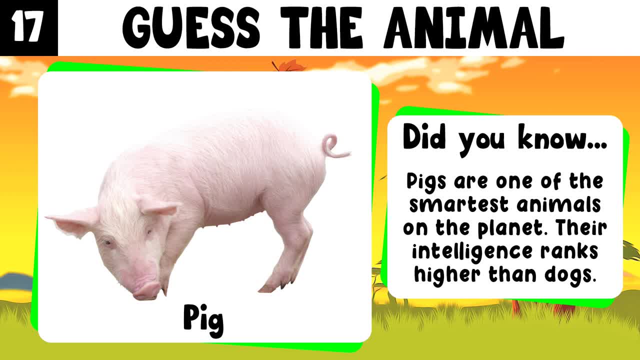 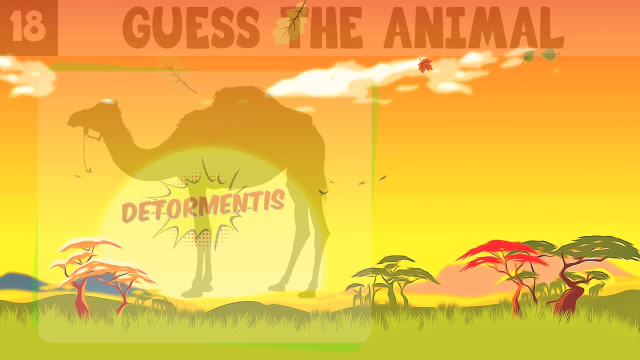 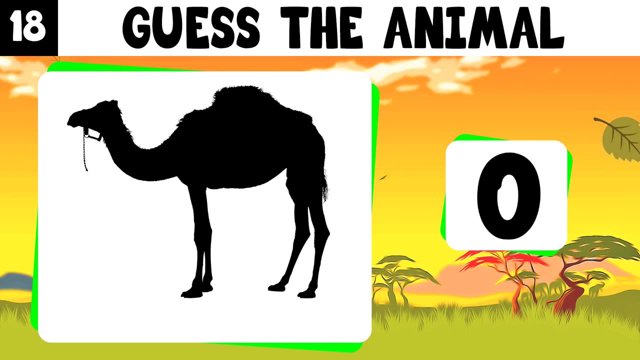 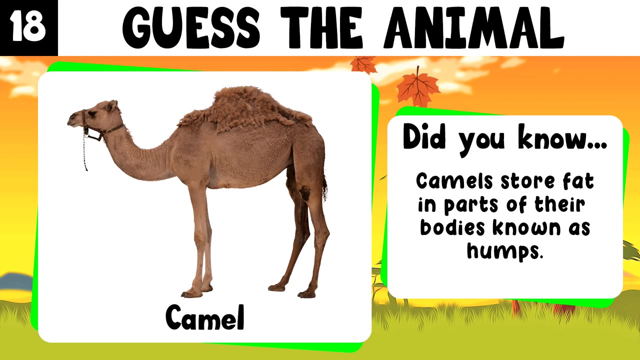 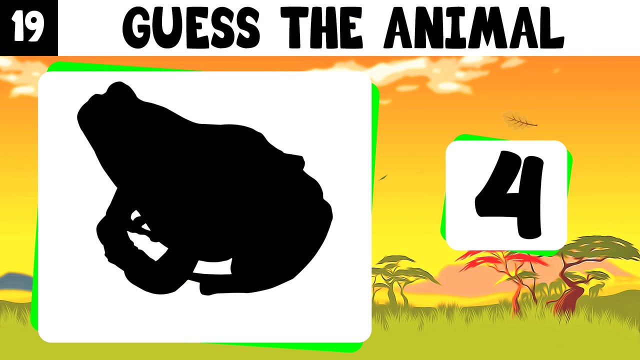 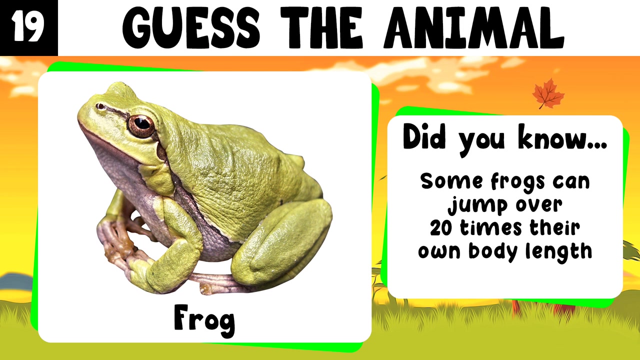 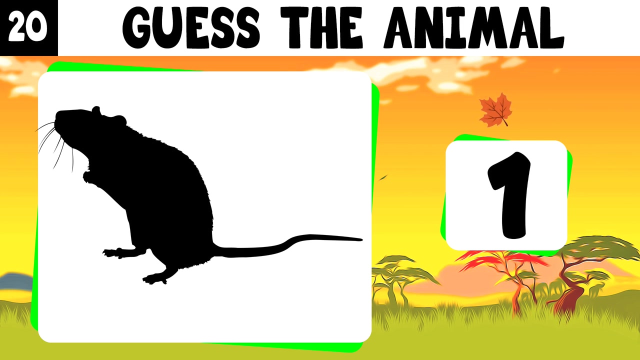 Pig: Pigs are one of the smartest animals on the planet. Their intelligence ranks higher than dogs. Camel Camels store fat in parts of their bodies known as humps. Frog- Some frogs can jump over 20 times their own body length. Rat: Certain types of rats can trade water for up. 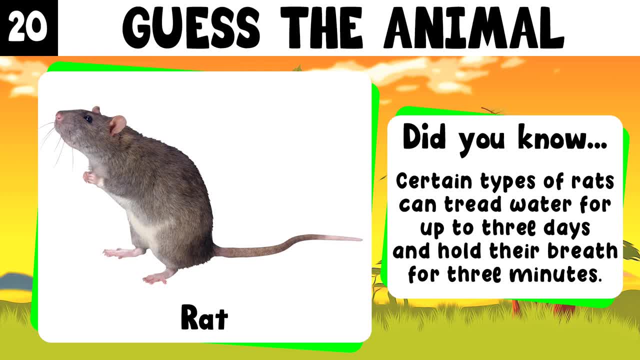 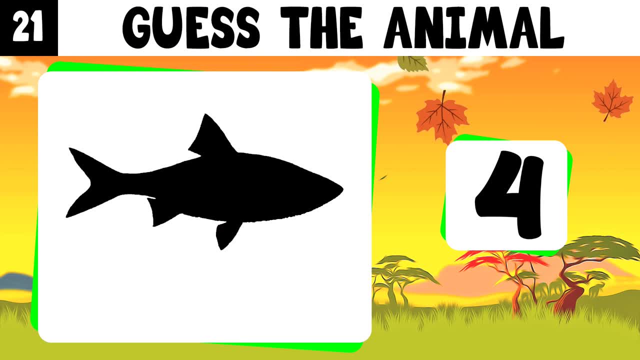 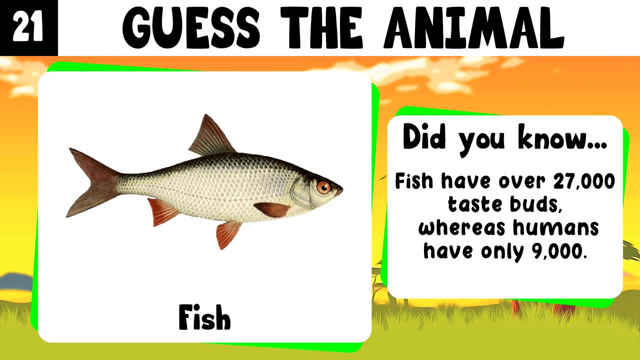 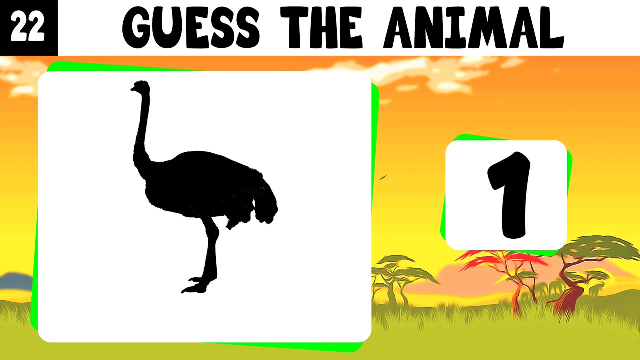 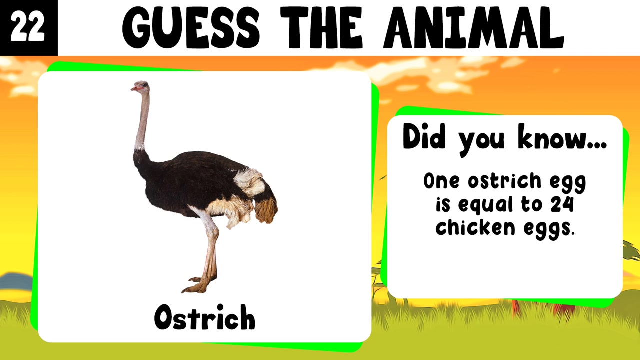 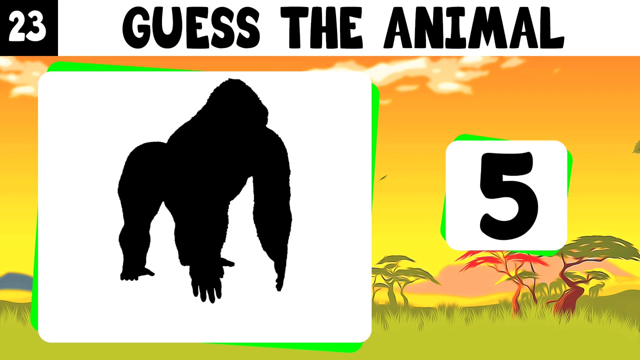 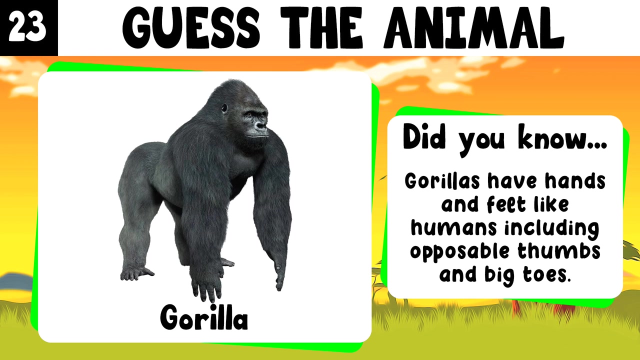 to three days and hold their breath for three minutes. Fish- Fish have over 27,000 taste buds, where humans have only 9,000.. Ostrich, Did you know? One ostrich egg is equal to 24 chicken eggs. Gorilla Gorillas have hands and feet like humans. 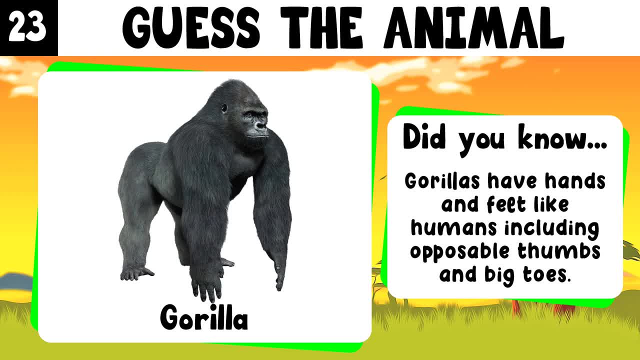 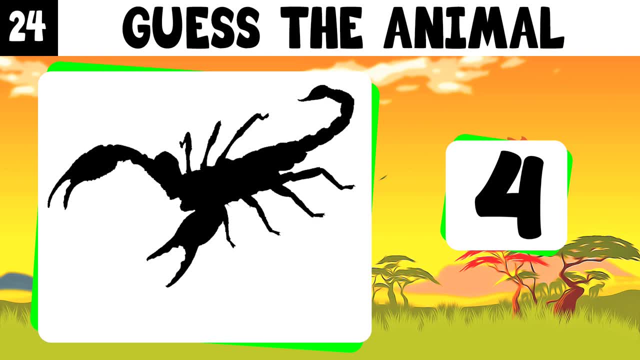 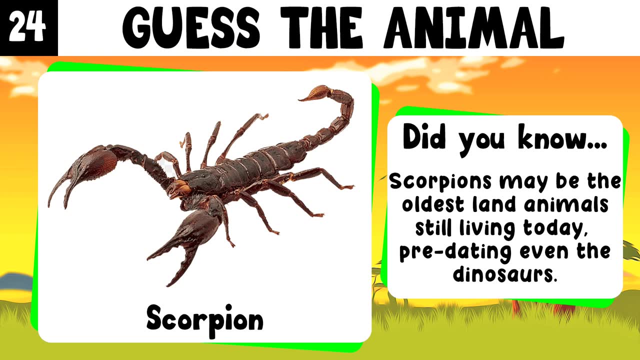 including opposable thumbs and big toes. There are more than 20 species of ostriches in the world, but only a few. Ostrich Dinosaur Scorpion. Scorpions may be the oldest land animal still living today, predating even the dinosaurs. 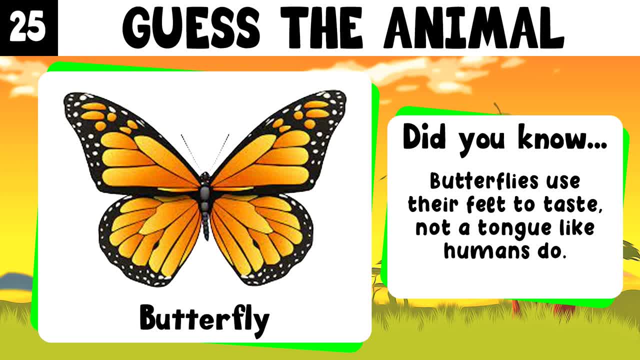 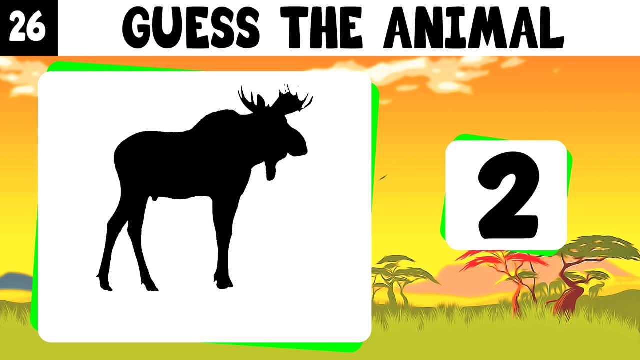 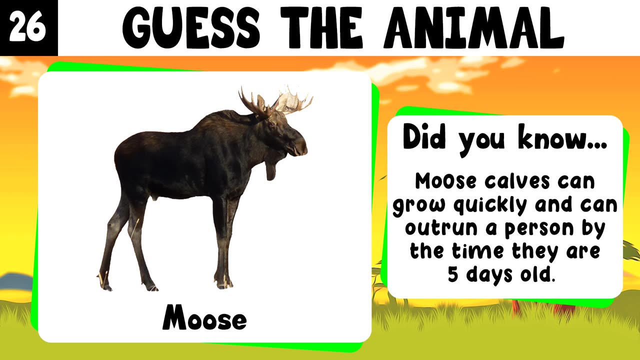 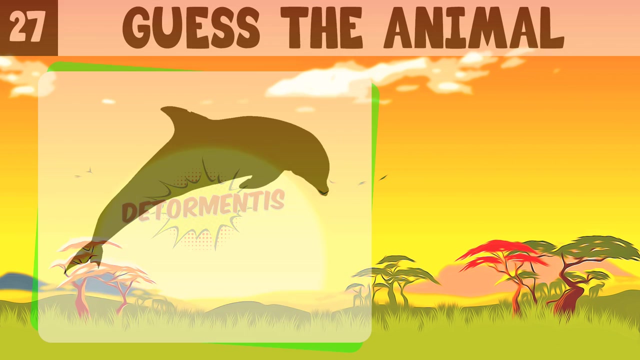 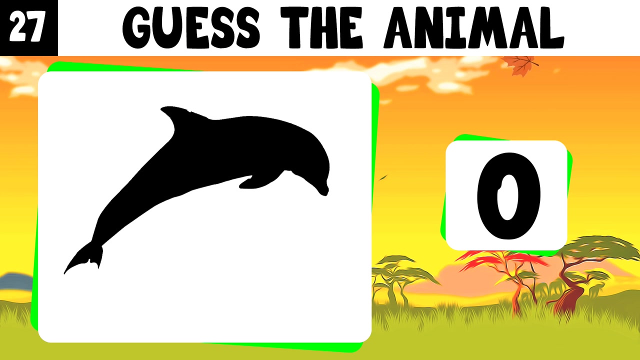 Butterfly. Butterflies use their feet to taste, not a tongue, like humans do Fish. conversely, they can bite when everyone is talking. Moose Moose calves can grow quickly and can outrun a person by the time they are 5 days old. Dolphin Dolphins can swim at 20 miles per hour and 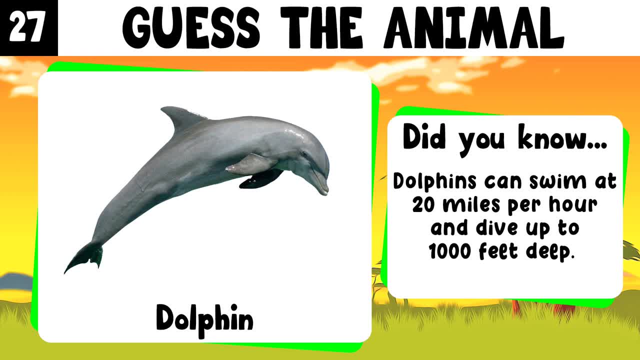 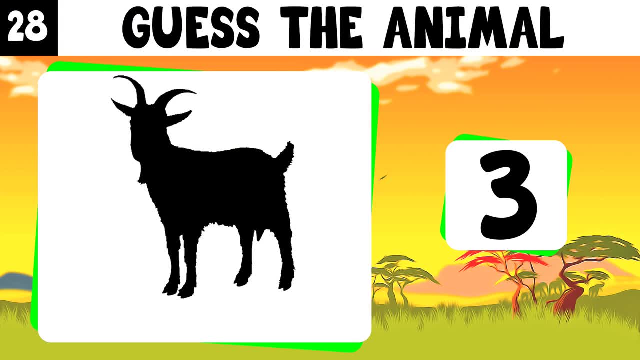 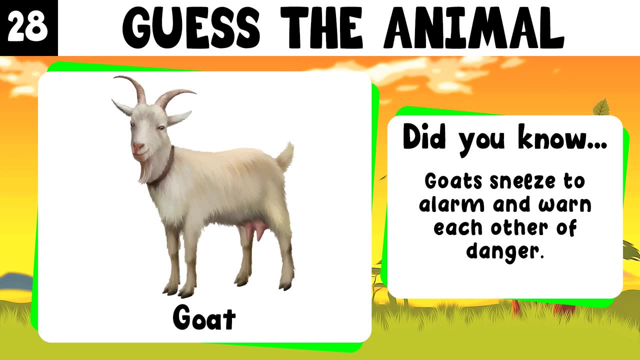 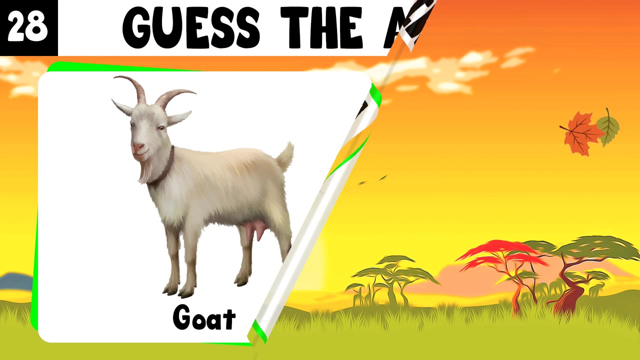 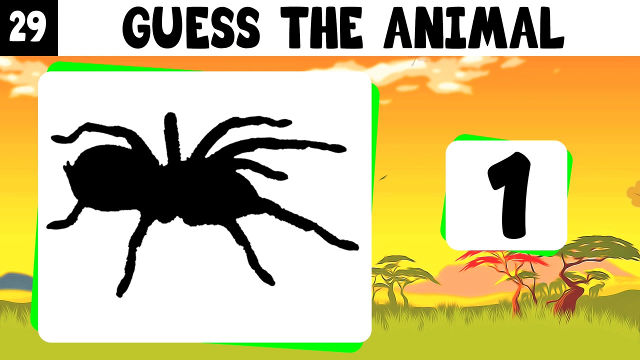 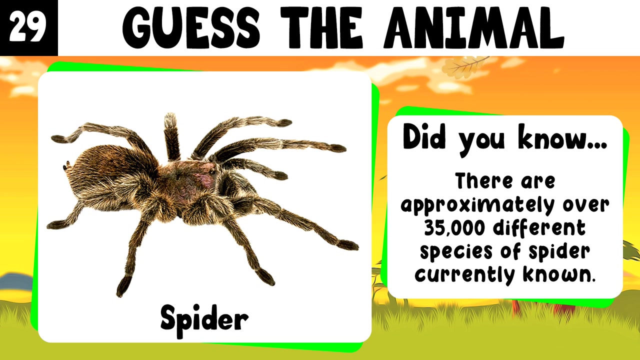 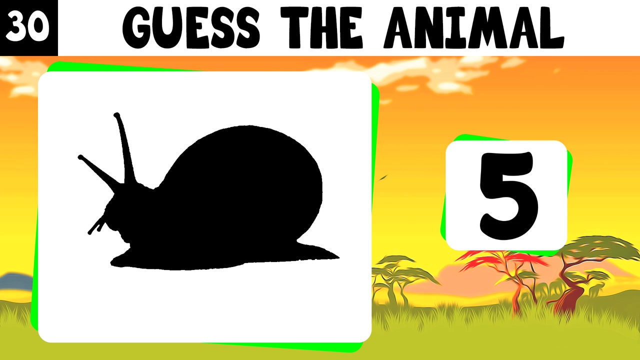 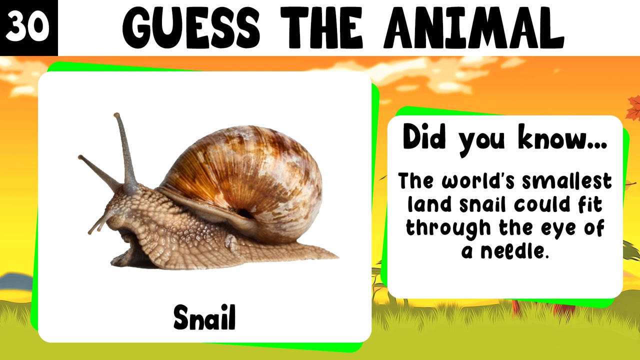 dive up to 1,000 feet. Goat- Goats sneeze to alarm and warn each other of danger. Coyote Spider: There are approximately over 35,000 different species of spider currently known. Snail: The world's smallest land snail could fit.